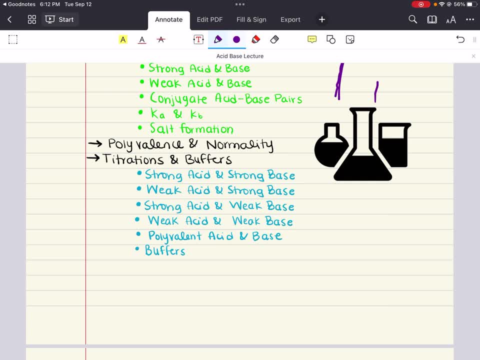 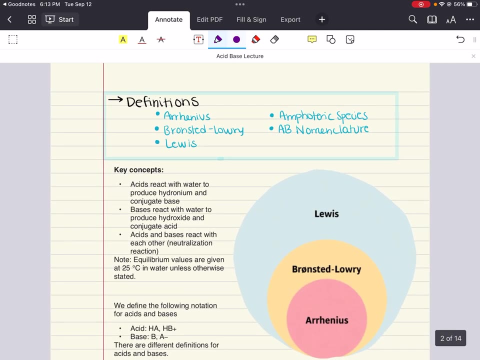 weak base. We'll also briefly touch on what titrations look for- polyvalent acids and bases, And then we'll end this chapter with a discussion on buffers. So let's go ahead and get started with that first objective, And I want to reiterate our 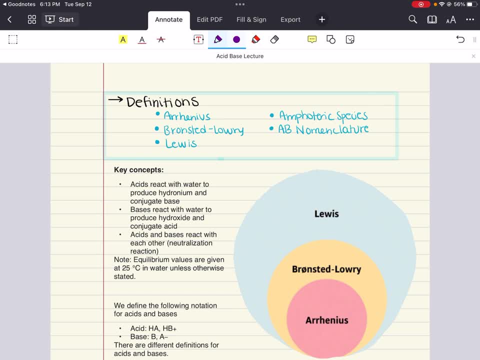 learning goals here. for this first objective, We want to define and then compare and contrast Arrhenius, Bronsted-Lowry and Lewis acids and bases, All right. and then we want to talk about amphoteric species and also determine if they're amphiprotic as well, And then we're going to learn. 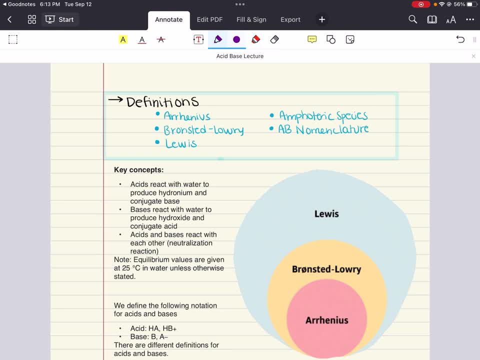 acid-base nomenclature. in addition, Now, over the last century, chemists have used different definitions to identify compounds as acids or as bases. Three definitions emerged each, with each one being more inclusive than the former. All right, we're going to start with that. 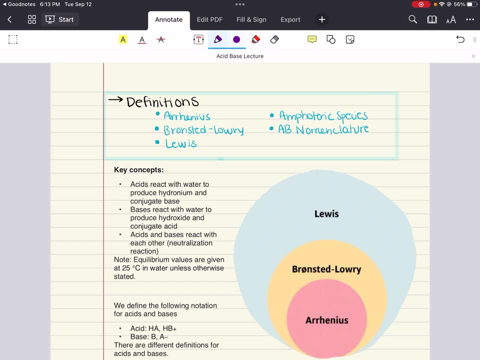 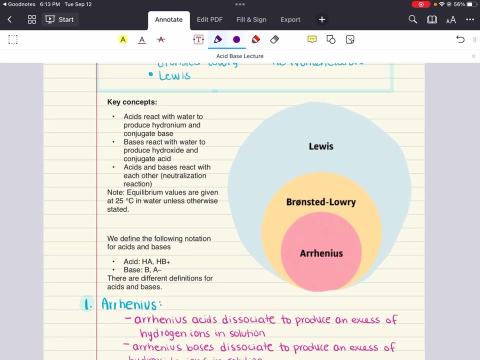 first definition, which is the Arrhenius definition. This is the first and most specific definition of an acid or base. An Arrhenius acid is defined as an acid that will dissociate to form an acid or a base. And that's the first definition. And then we're going to. 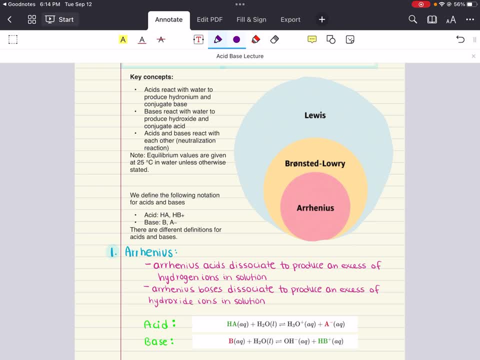 look at the second definition, which is an acid that will dissociate to form an excess of H plus in solution. So hydrogen ions in solution And an Arrhenius base will dissociate to form an excess of OH minus or hydroxide in solution. Now these behaviors are generally limited to aqueous acids. 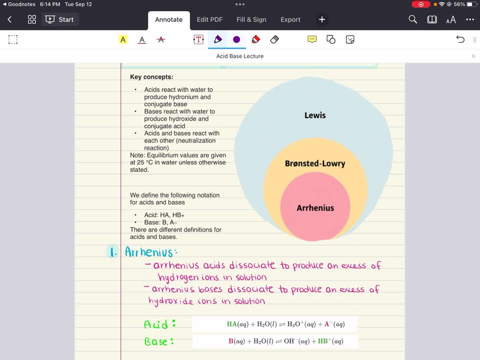 and bases. The thing is, though, Arrhenius acids and bases are very easily identified. Acids contain a hydrogen at the beginning of the formula, So hydrochloric acid, HCl, nitric acid, HCl and hydrochloric acid, And then we're going to look at the second definition. 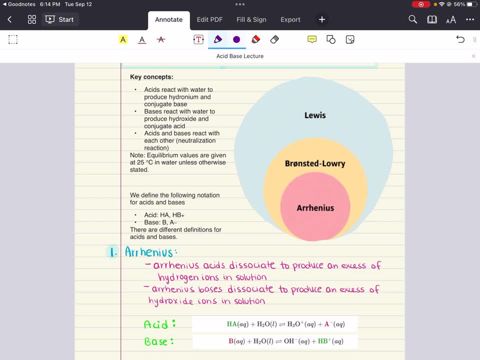 HNO3, sulfuric acid, H2SO4, and so on, And bases. they're also easy to identify because they contain OH at the end of their formula, So sodium hydroxide, NaOH, calcium hydroxide. 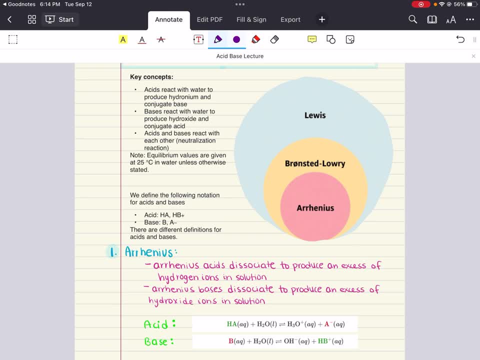 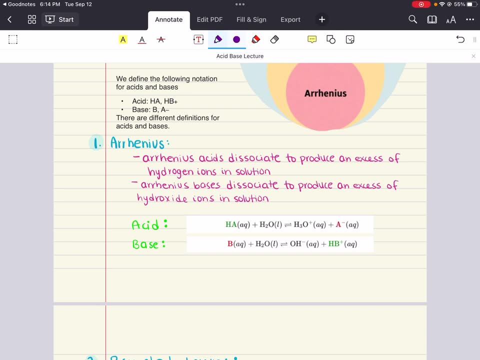 CaOH2, and so on and so forth. Now any mention of the Arrhenius definition on MCAT test day is going to be likely. in comparison to other definitions of acids, The Arrhenius definition is by far the most restrictive: The Branstad-Lowry and the Lewis. 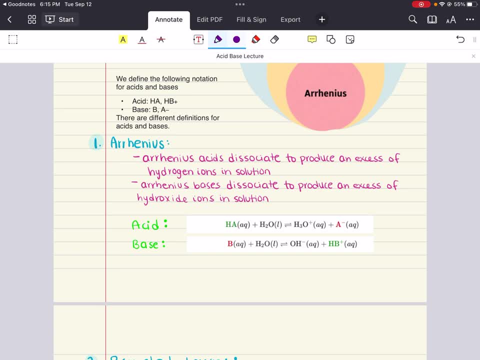 definitions definitely predominate on the MCAT. So that's a good thing to know, but still familiarize yourself with the Arrhenius definition, All right. So again, an Arrhenius acid will dissociate to produce an excess of hydrogen ions And an Arrhenius base will dissociate to produce an. 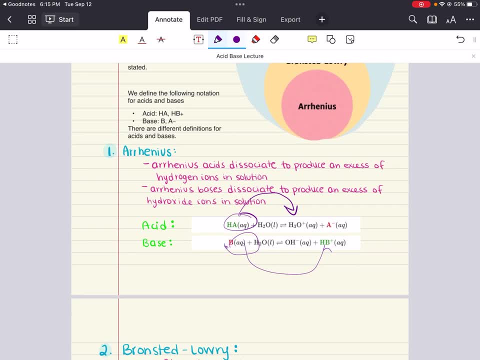 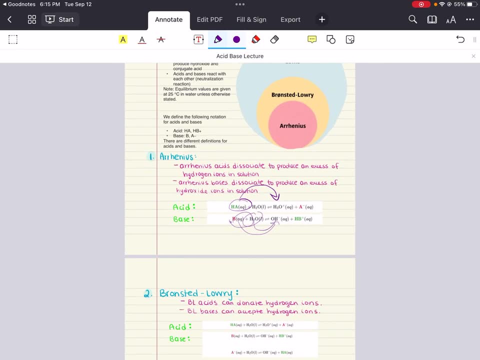 excess of hydrogen ions. So again, an Arrhenius acid will dissociate to produce an excess of hydroxide ions in solution. Sorry, the arrow should be pointing this way. Awesome. I don't know what's wrong with my pen. I think I might need to get a new one. Regardless, that's the. 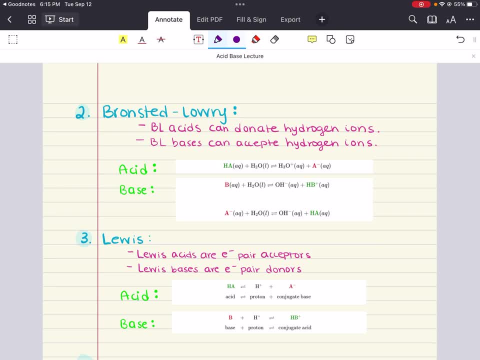 Arrhenius acid and base definition. Next up, all right, is Branstad-Lowry acids and bases. These are more inclusive, All right. So Branstad-Lowry acid: this is going to be a species that donates hydrogen ions And this is going to be a species that donates hydrogen ions, And this is going to. 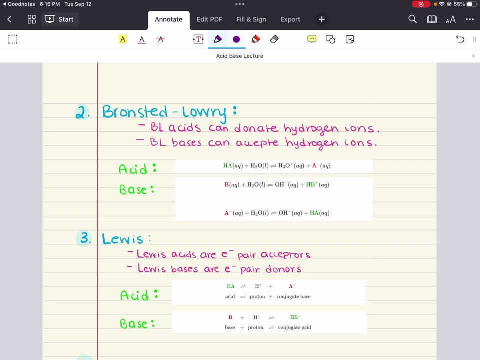 while Branstad-Lowry base is a species that accepts those hydrogen ions. The advantage of this definition, especially over the Arrhenius one, is that it's not limited to aqueous solutions, So, for example, hydroxide ammonia, fluoride ions. there's all Branstad-Lowry bases because each has 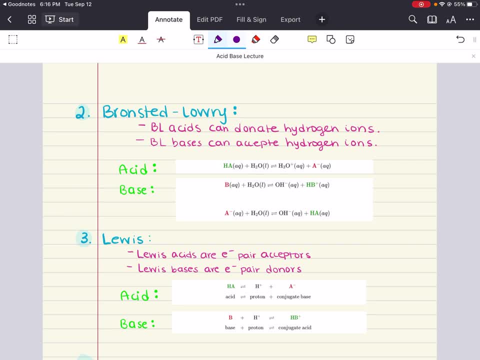 the ability to accept a hydrogen ion. However, neither ammonia or fluoride ions can be classified as Arrhenius, So this is definitely a more inclusive definition of acids and bases. All right, Fantastic. So again, acids can donate hydrogen ions. Notice how this acid is donating a hydrogen ion to water here. 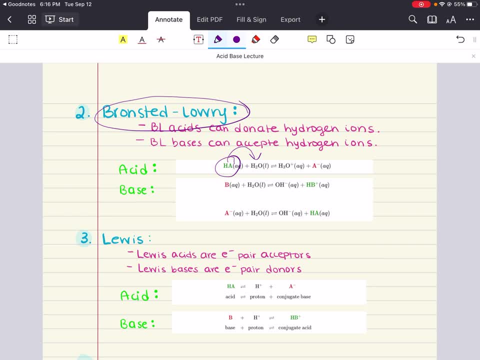 in this example, All right. And then Branstad-Lowry bases can accept hydrogens- All right. So you'll notice that this base right here accepts a hydrogen from water- All right, To result in hydroxide being formed, NHA, All right. Fantastic Now, according to both. 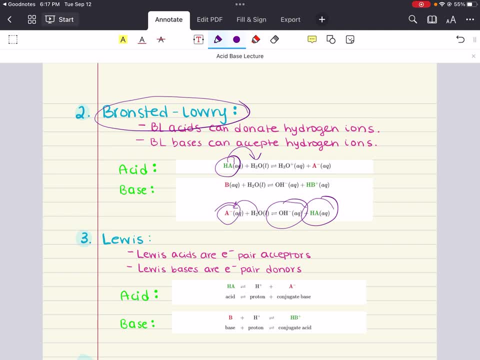 of these definitions, Arrhenius and Branstad-Lowry, there is only one way for a species to be an acid, and that's to produce hydrogen ions. Then the only difference between the two definitions for acids are the requirement of hydrogen ions. So the only way for a species to be an acid, and that's to 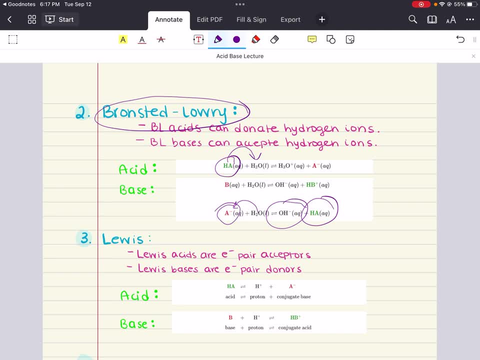 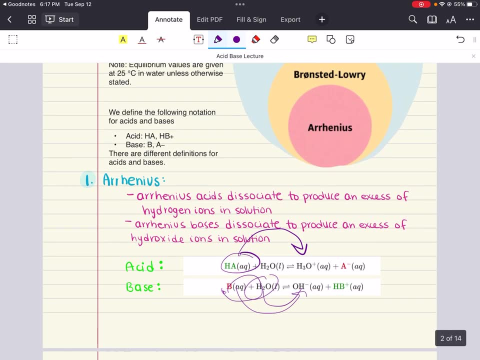 produce hydrogen ions. So in the Arrhenius definition water is not considered an acid. So in the Arrhenius definition, all right. in the Arrhenius definition, Arrhenius acids dissociate to produce an excess of hydrogen ions in solution. According to this definition, water is not. 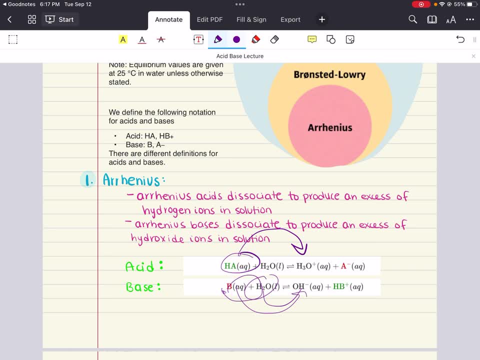 considered an acid. It does not produce an excess of hydrogen plus ions in solution. Water is, on the other hand, a Branstad-Lowry acid because it is a todosac, So would the acid in water is an acid in solution. 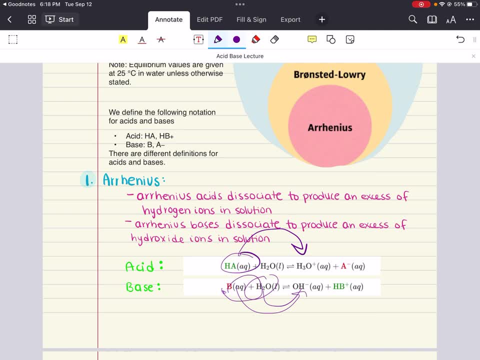 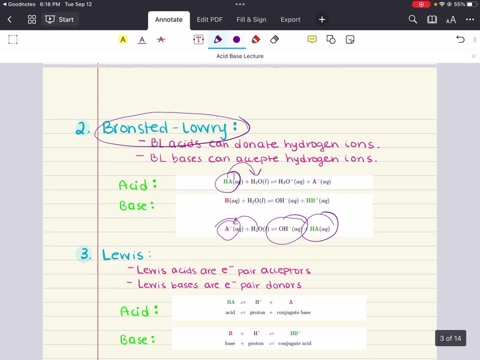 No, Okay. No, it is able to donate a proton to other species. So that's an important distinction to make between the two. Now, Bronsted-Lowry acids and bases- they always come in pair because the definition requires the transfer of a proton from the acid to the base- is called conjugate acid-base pairs. 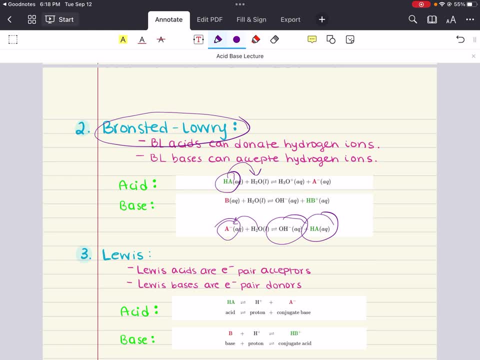 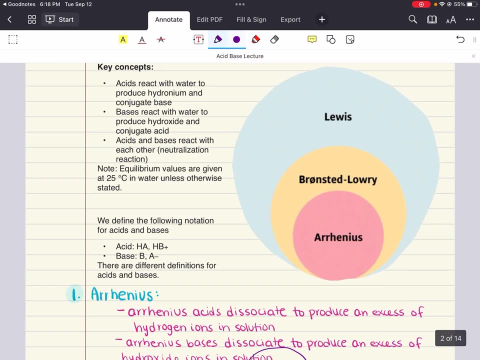 We're actually going to talk about them in more detail shortly. Now something else to keep in mind: this figure right here displays a very important concept. all right, And we're going to come back to it again, even when we define Lewis acids and bases. But what you realize here? 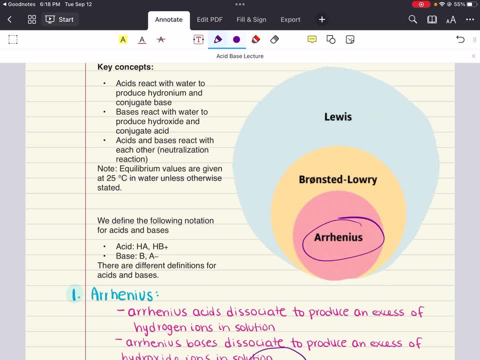 is that every Arrhenius acid or base can also be classified as a Bronsted-Lowry acid or base. all right, And that's because, again, Bronsted-Lowry definition of acids and bases is more inclusive. Now, something else we'll notice is that every Bronsted-Lowry acid or base can: 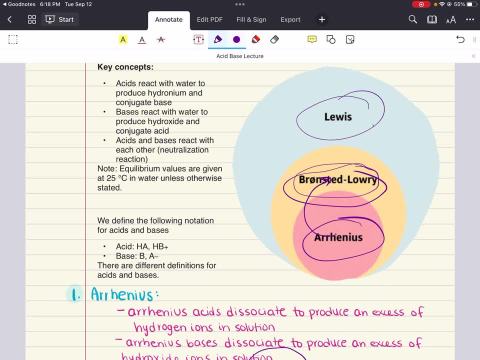 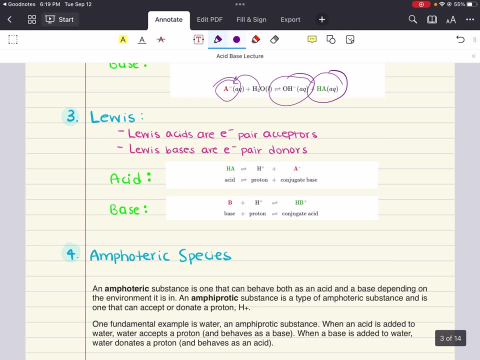 also be classified as a Lewis acid or base, also because it's even more inclusive. all right, Now here's the catch: This logic doesn't always work the other way, so be careful With that. let's discuss Lewis acids and bases At approximately the same time that Bronsted. 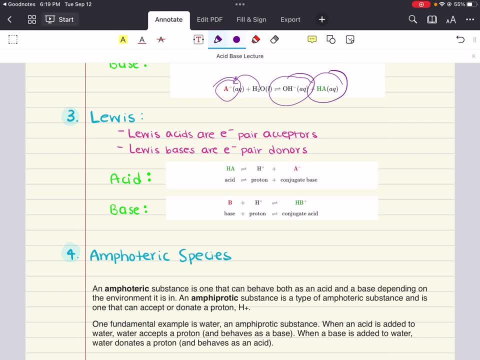 and Lowry's publication about their definition of acids and bases. Gilbert Lewis also proposed a definition of acids and bases. He said acid is going to be defined as an electron pair acceptor and a Lewis base is defined as an electron pair donor. all right, And there's an intuitive approach really to understanding. 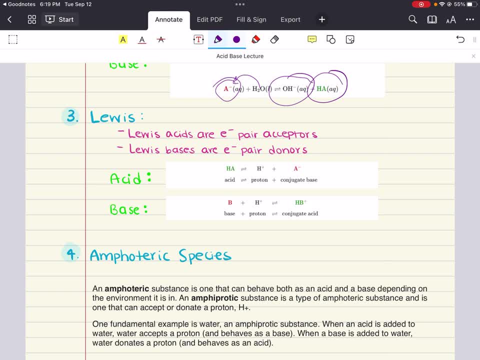 the difference in the definitions we have discussed so far. And that is well. the Lewis definition relies on a behavior that is not vastly different from the Bronsted-Lowry interactions. The only difference really is just the focus. So for Bronsted-Lowry, 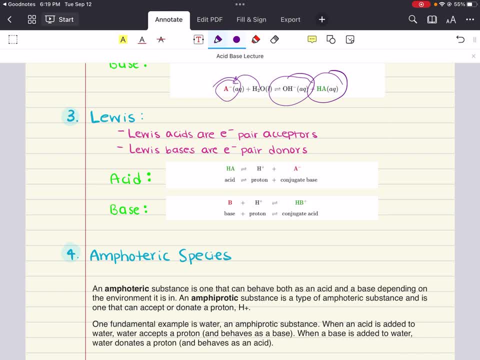 acids and bases, we follow the exchange of the hydrogen ion, which is essentially just a naked proton In the Lewis definition. the focus of the reaction is no longer on the proton, but instead the electrons forming the coordinate covalent bonds. all right, Again, note that the Lewis 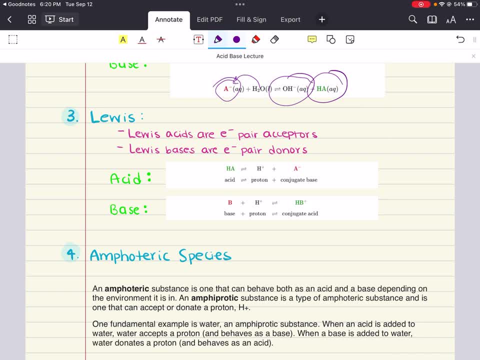 definition is the most inclusive. Every Arrhenius acid is also a Bronsted-Lowry acid and every Bronsted-Lowry acid is also a Lewis acid. All right, And likewise for the bases, And be careful. the opposite is not always true. 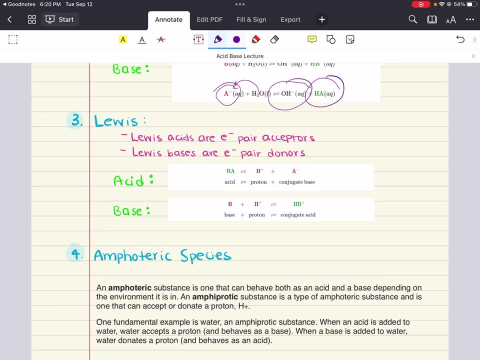 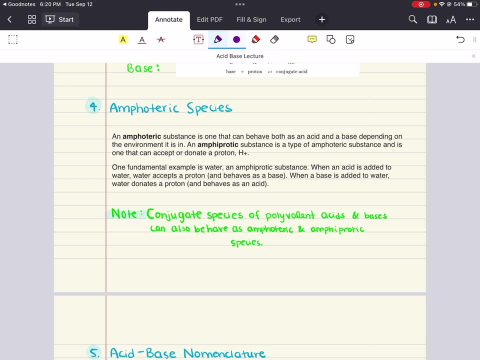 all right, Fantastic. So those are our definitions of acids and bases. Let's discuss amphoteric species. An amphoteric species is one that reacts like an acid in a basic environment and like a base in an acidic environment. So in the Bronsted-Lowry sense, an amphoteric species. 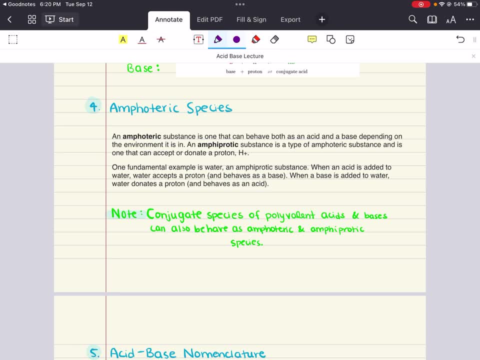 can either gain or lose a proton, Making it amphiprotic as well. On the MCAT, water is the most common example of this. When water reacts with a base, it behaves as an acid All right, So that's an important thing to note When 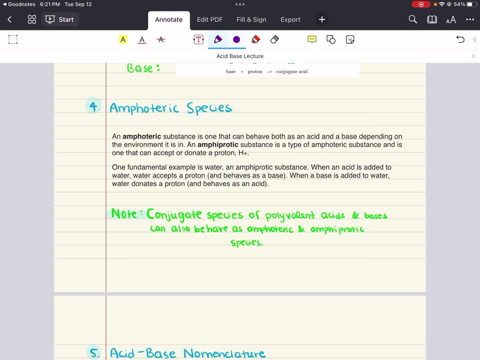 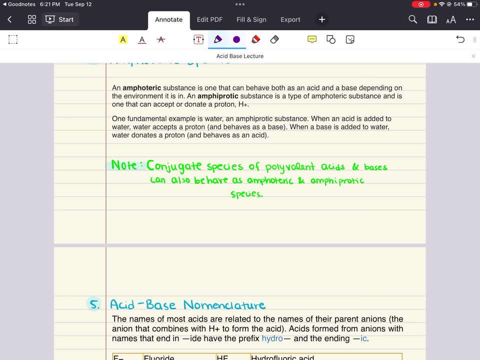 water reacts with a base, it behaves as an acid. And then when water reacts with an acid, it behaves like a base. All right, So with that let's kind of demonstrate that When water reacts with an acid base, it behaves as an acid. We can see that if we write H2O and it reacts with a base, we're going. 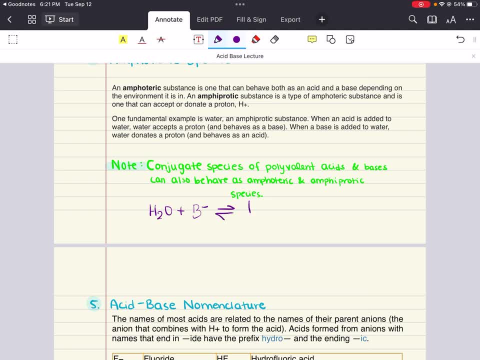 to denote our base B minus. all right. In this environment, water acts like an acid. It donates a hydrogen to the base and we have HB that forms and OH minus, all right. So this is when water reacts with a base. So water plus base, all right. Water acts like an acid, Cool. Now what about? 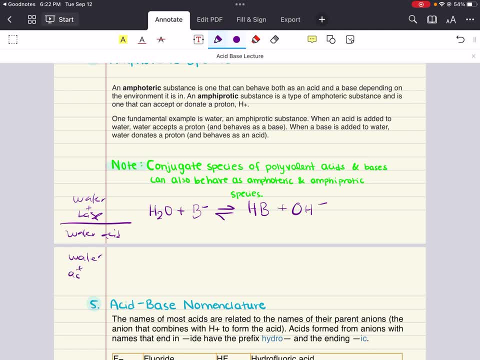 water. What if water reacts with an acid? all right. What if water reacts with an acid? So here's an acid, here's water, all right. What happens is that the acid gives the water its hydrogen, so we form what is called the hydronium ion plus A minus. So not plus A minus. There we 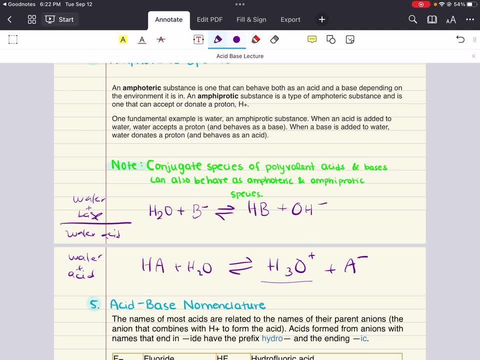 go. So when a water reacts with an acid it B, It behaves as a base. all right, Now water amino acids, even partially deprotonated polyprotic acids, are common examples of amphoteric and amphiprotic substances, Metal oxides and 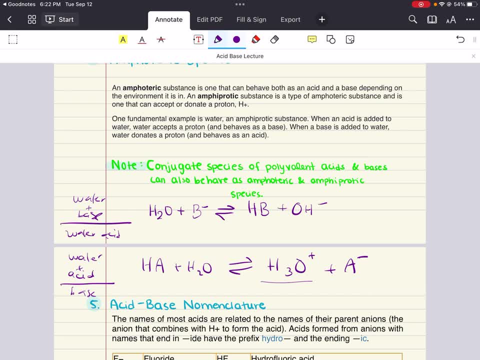 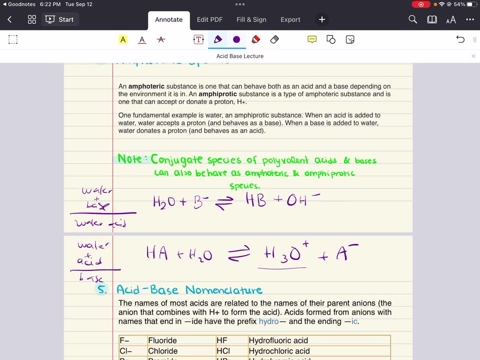 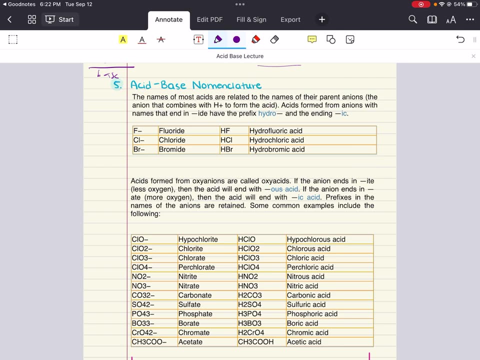 hydroxides are also considered amphoteric, but not necessarily amphiprotic, because they do not give off protons- Fantastic. Now the last thing we want to cover in objective one is, of course, acid base nomenclature. The names of most acids are: 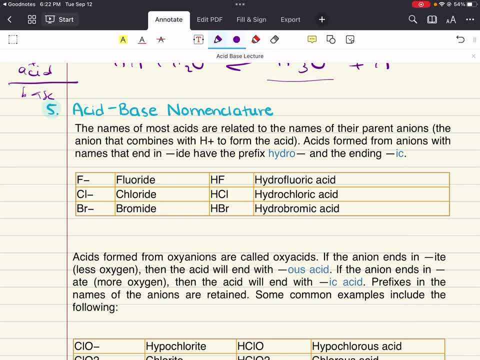 going to be related to the names of their parent anions, the anion that combines with H plus to form the acid. So acids formed from anions with names that end in. I have the prefix hydro and the ending ik, all right, So let's go over this. If you have fluoride ions. 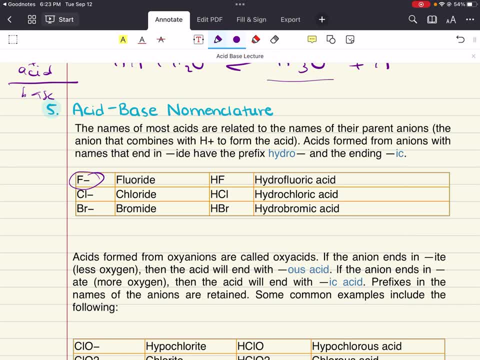 the acid form. if this was an acid form, it would be called hydrofluoric. ends with ik now instead of ide. acid, All right. what about chloride? All right. the acid form: hydrochloric acid. Notice how the ide is replaced with an ik. There's a hydro to start off that word. 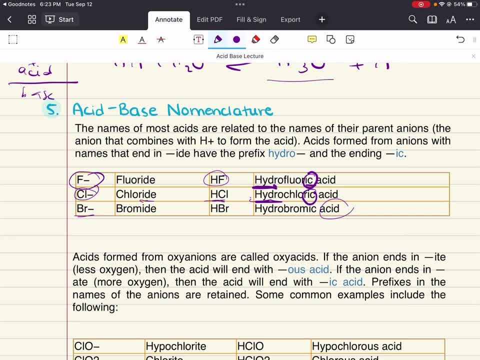 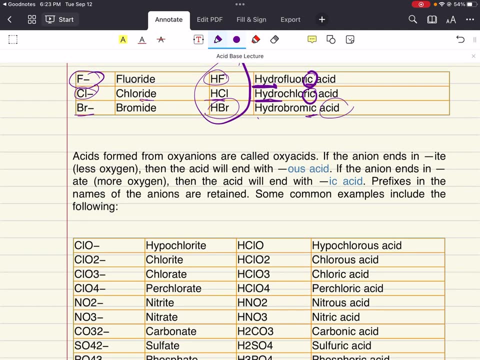 all right. And then you end off with acid. What about bromide? All right. acid form, hydrobromic acid- All right. so these are three acids. you should definitely know the names, of all right. Acids formed from oxyanions. they're called oxyacids. If the anion ends in ite, then the 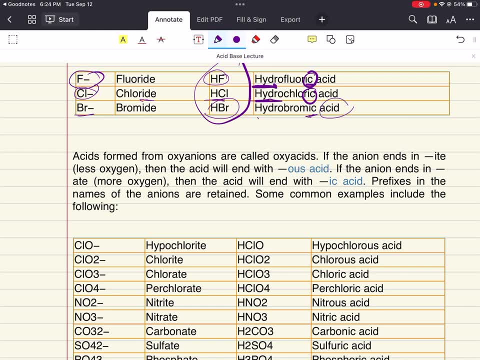 acid form will end with alice acid, And if the anion ends in ate, then the acid will end with ik acid. all right, Prefixes in the names of the anions are retained, And here we have a lot of examples. So here, 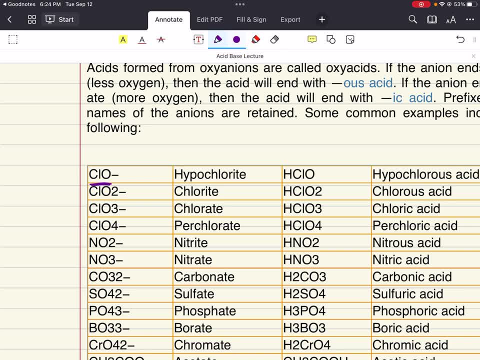 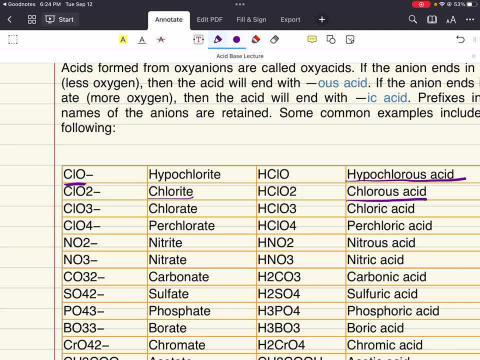 this is hypochlorite acid- all right, This is chloride. This is hypochlorous acid- all right, This is chlorous acid. Chlorate chloric acid- This is always hard for me to pronounce. Perclorate- all right, Percloric acid. Nitrite nitrous acid: Again, remember the hint we just 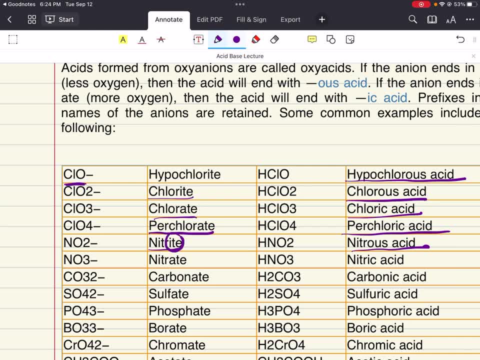 said: If the anion ends in eye, all right. This, for example, this: ions ends in I, All right. Then the acid will end with O. is acid just like we see here? nitrous acid, All right. Nitride, the acid form, nitrous acid, All right. Notice how this one here right. 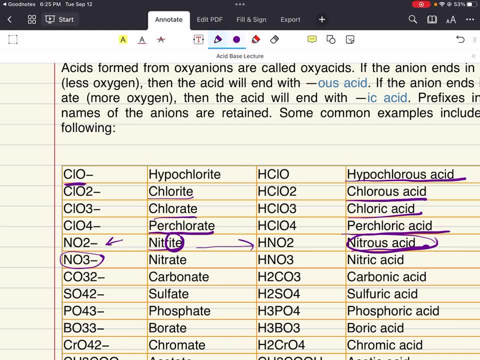 though this anion ends with A-T, A-T, nitrate, All right. That means the acid form of this will end in I-C acid. So this is nitrate. That acid form is nitric acid, All right, And so on. 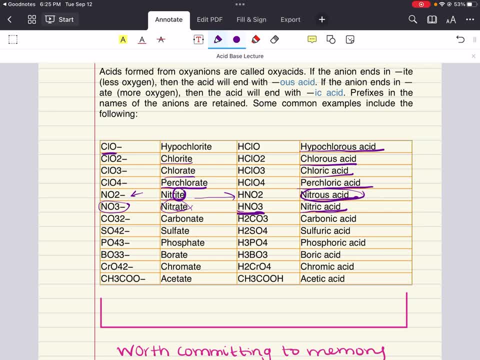 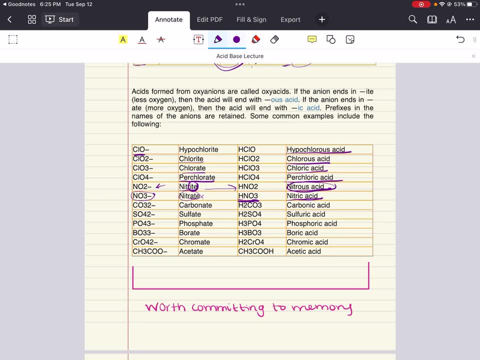 and so forth. for all of these examples, All right, My recommendation: if you're taking advice from me, these are worth committing to memory. All right, Whether you use the hint. all right that anions that end in I. all right, their acid will end in O-S acid. Their name for the acid will end in O-S. 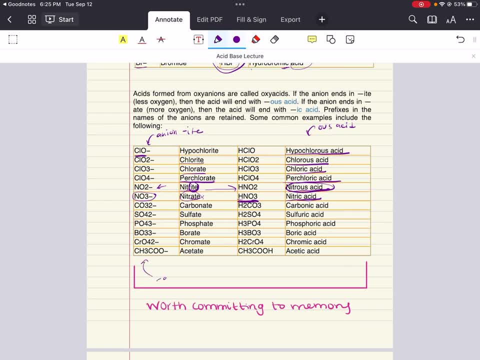 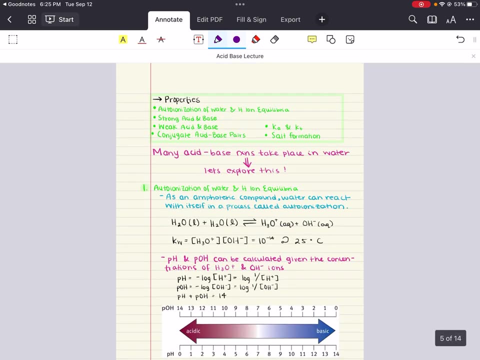 acid, And if the anion ends in A-T, its acid form is going to end in I-C acid. All right, Nevertheless, I think it's really important that you familiarize yourself with these names. All right, With that, we can move into the second objective now. Here we're going to cover properties of acids and bases. 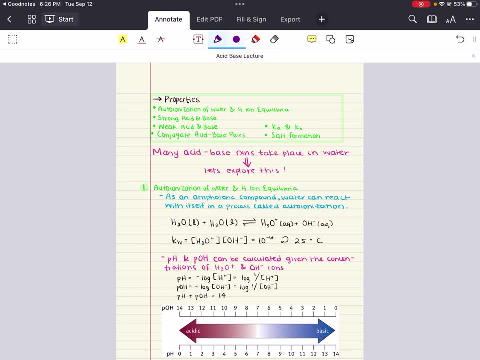 And here are the learning goals. Okay, We want to learn how to predict the behavior of an acid or base in water. All right, We want to be able to apply the mathematical relationships between pH, pOH and ion concentration. We want to recall the mathematical 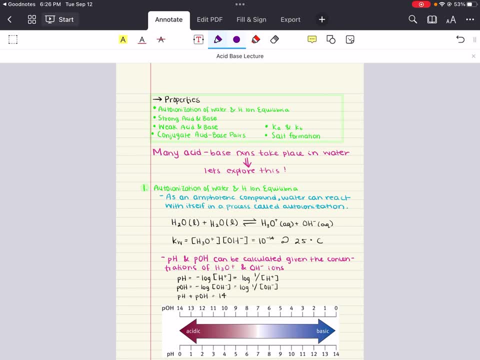 relationships between Ka Kb and Kw, All right. And we also want to be able to determine concentration of hydrogen ions given either molarity and or Ka Kb values. All right. So those are kind of the goals for this objective. The first topic of conversation here is auto. 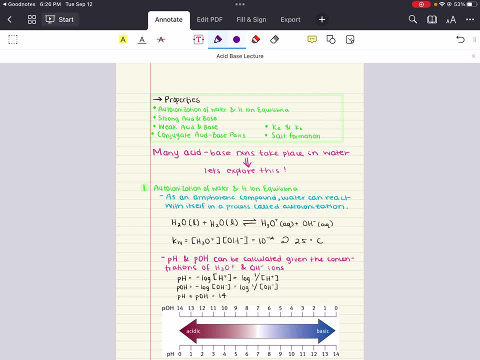 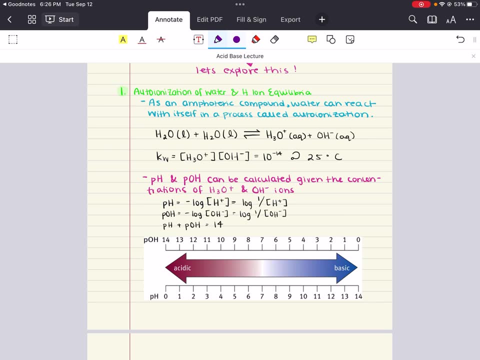 ionization of water and hydrogen ion equilibria. All right Now, because many acid-base reactions take place in water, especially on the MCAT, it is going to be very important to understand the behavior of acidic and basic compounds in water. Only then can one really fully appreciate the meaning and significance of such terms. 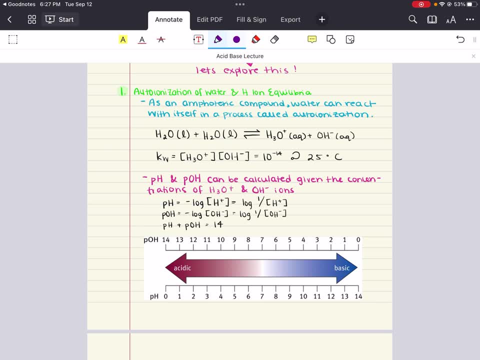 like strong acid, weak acid, strong base, weak base or even the measurements of pH and pOH. Now, as we described earlier, water is an amphoteric species, So in the presence of a base it reacts as an acid, And in the presence of an acid it reacts as a base, Now as an amphoteric. 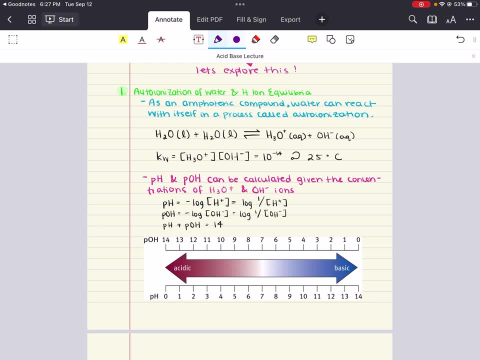 compound. water can actually react with itself in a process called auto ionization. All right, As seen here in this reaction. look at water reacting with water. All right, We have this auto ionization reaction: One water molecule donates a hydrogen ion to another water molecule. 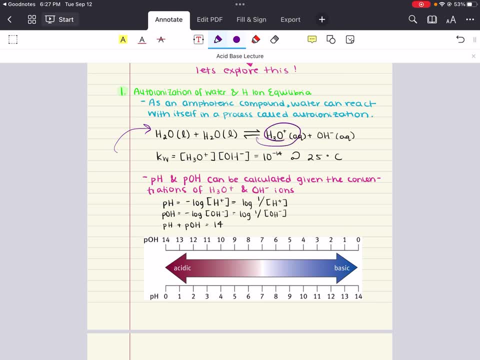 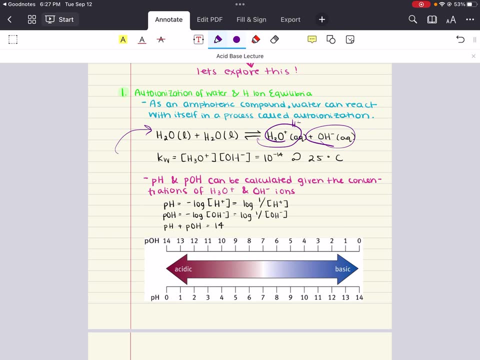 The hydrogen ion and the hydroxide ion. Now many general chemistry courses depict the hydrogen simply as H plus sometimes, rather than H3O plus, So just be cautious of that in case it's written in that format. Nevertheless, auto ionization of water is a reversible reaction, And so we can. 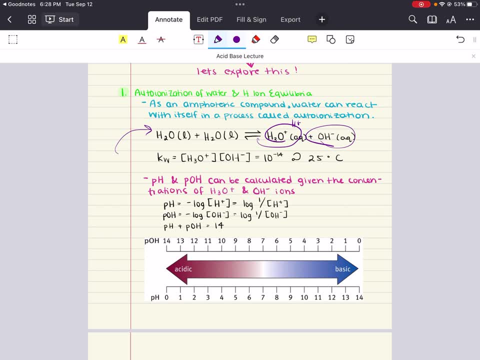 write a water dissociation reaction, And so we can write a water dissociation reaction And so we can translate that into a water dissociation constant. All right for this process. So for pure water at 298 Kelvin, the water dissociation constant all right is going to be all right. 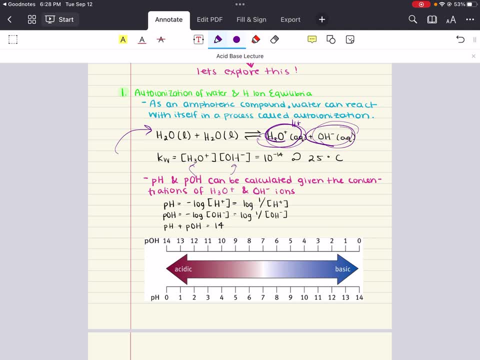 just your products. So hydronium ions concentration and hydroxide ion concentrations, Remember, our equilibrium constants only take into account aqueous species. So since these waters in the reactant sides are liquids, they're not accounted for, And this has been. 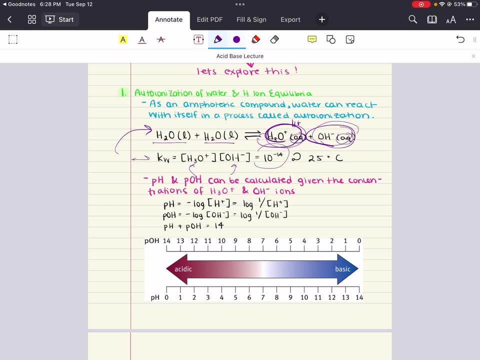 experimentally determined to be 10 to the minus 14.. All right, 10 to the minus 14.. And this is again at 25 degrees Celsius or 298 Kelvin. All right, Now, each mole of water that autoionizes. 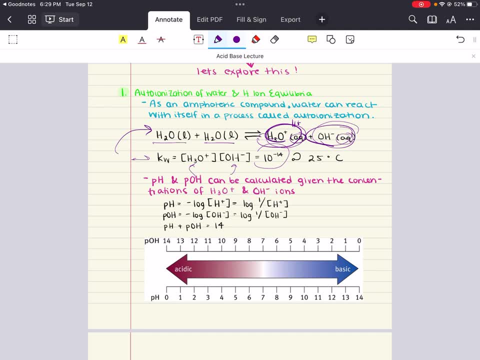 produces one mole each of hydrogen ions and hydroxide ions. So the concentration of the hydrogen ions and the hydroxide ions are always equal in pure water at equilibrium. All right. And so if we know what the water dissociation constant is, all right, and we know that fact. 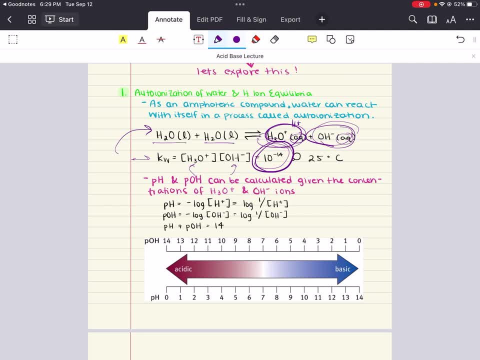 that we just stated that each mole of water that autoionizes produces one mole each of hydrogen ions and hydroxide ions. All right, Then. the concentration of the hydrogen ions and the hydroxide ions are always equal in pure water at equilibrium, And so that means 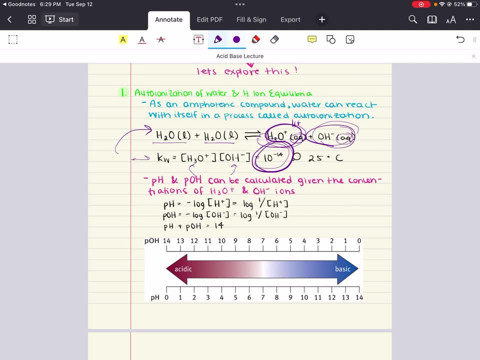 the concentration of each of the ions in pure water. This is 10 to the minus seven molar. All right, And this is 10 to the minus seven molar. And just as a reminder, KW, or the water dissociation constant, is an equilibrium constant. So, unless the temperature of the water 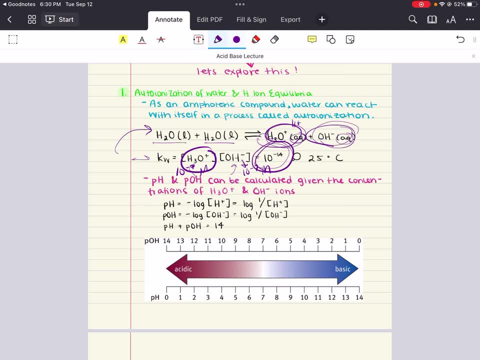 is changed, the value for KW cannot be changed, All right, And so the product of the concentrations of the hydrogen ions and the hydroxide ions in an aqueous solution at 298 Kelvin must always equal 10 to the minus 14.. Of course, if you change the temperature, 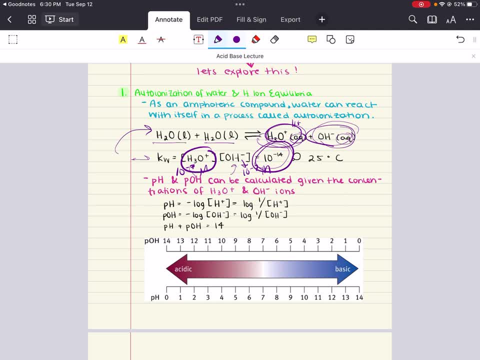 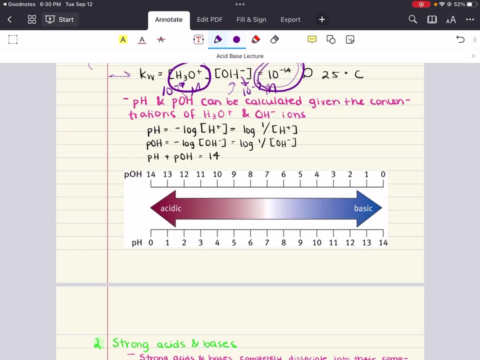 then the value of KW changes. Now, at temperatures above 298 Kelvin, KW will increase. This is a direct result of the endothermic nature of the autoionization reaction. Now what we also want to talk about and introduce is the scale used in measuring concentrations of hydrogen ions. 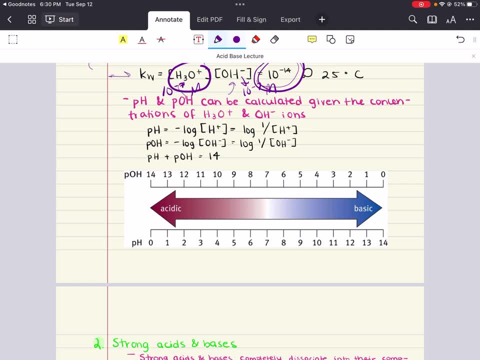 and hydroxide ions in different acid based solutions, The concentrations of hydrogen ions and hydroxide ions in aqueous solutions. they can vary differently, making the ranges of measurements on a linear scale actually pretty unmanageable. All right, The concentration scales. 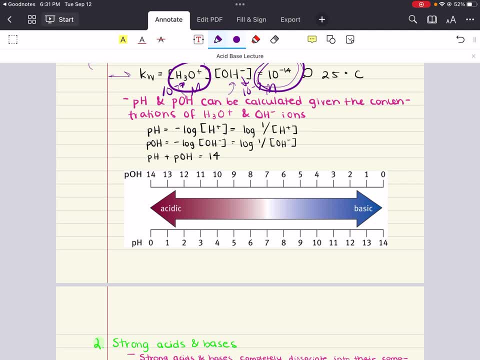 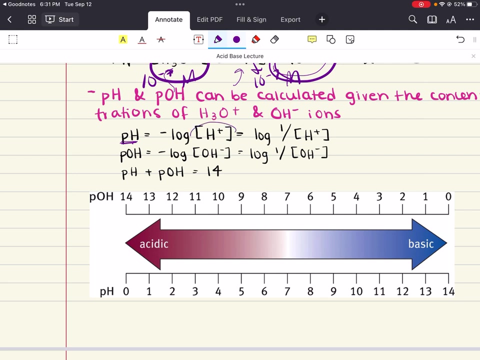 for acidic and basic solutions are actually condensed into something more manageable through expression in logarithmic terms. These log scales are the pH and the pOH scales for the concentrations of hydrogen and hydroxide ions respectively. All right, And we can see all right that pH is the negative log of the hydrogen ion. 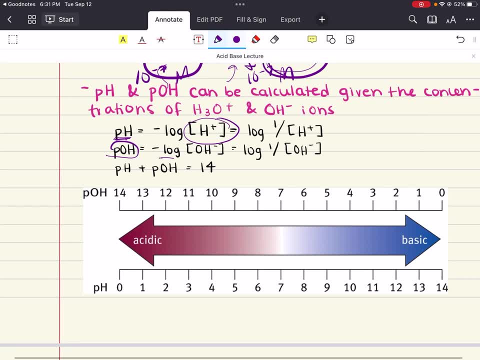 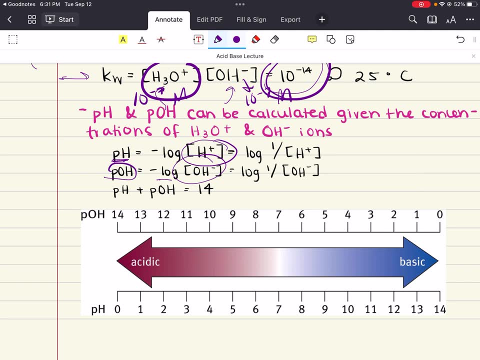 concentration, and pOH is the negative log of the hydroxide ion concentrations. Another important thing to keep in mind is that the sum of pH and pOH is equal to 14.. All right, We have our acid-base scale here. All right, It's a scale of 0 to 14.. For an aqueous solution at 298 Kelvin. 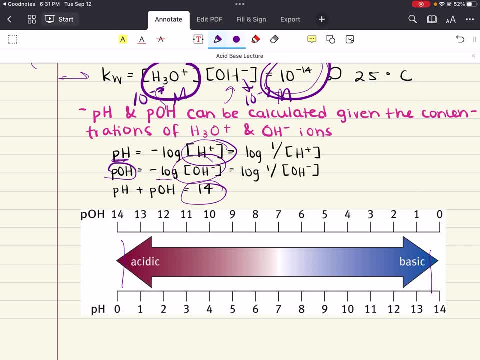 a pH less than 7,. so if our pH is less than 7 and our pOH is greater than 7,, all right or sorry. if our pH is less than 7 or our pOH is greater than 7,, all right. 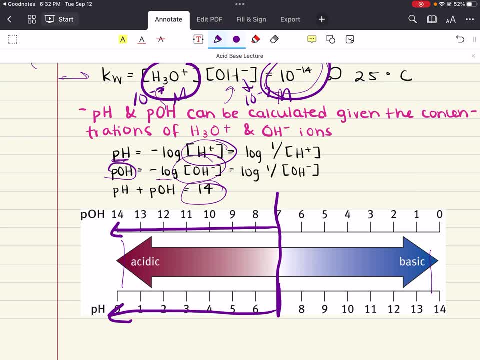 that indicates a relative excess of hydrogen ions and the solution is acidic. Okay, What about a pH greater than 7 or a pOH less than 7? What does that mean? That indicates a relative excess of hydroxide ions and the solution is basic: A pH and pOH. 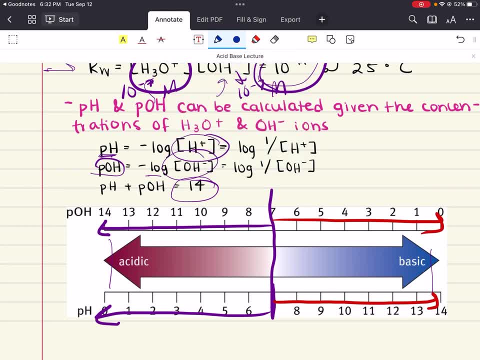 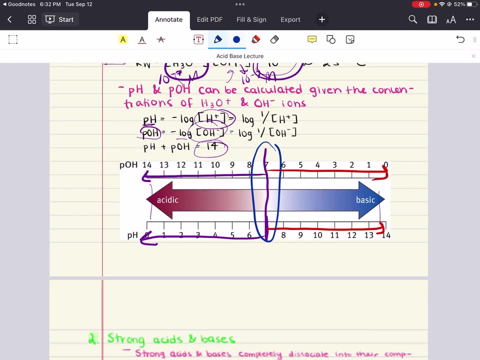 that's equal to 7, all right. if it is equal to 7 for both scales, all right. that indicates equal concentrations of hydrogen and hydroxide ions, resulting in a neutral solution. Fantastic. With that we want to talk about strong acids and 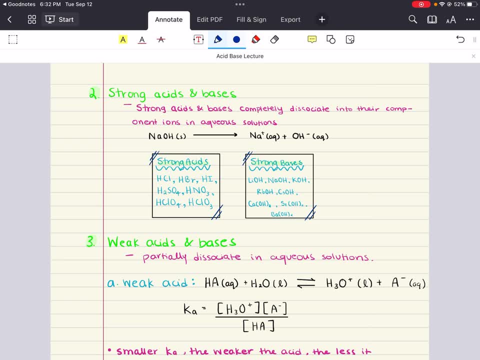 bases, and then weak acids and weak bases. So strong acids and strong bases, they completely dissociate into their component ions. I'm sorry if I sound a little congested. I am getting sick, All right, So just forewarning you. Anyways, strong acids and bases. 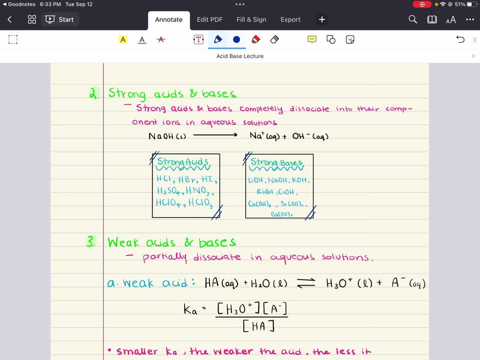 they completely dissociate into their component ions in aqueous solution. So, for example, when sodium hydroxide is added to water, the ionic compound dissociates, all right, dissociates into sodium cations, hydroxide and ions. Now virtually no undissociated strong acid. 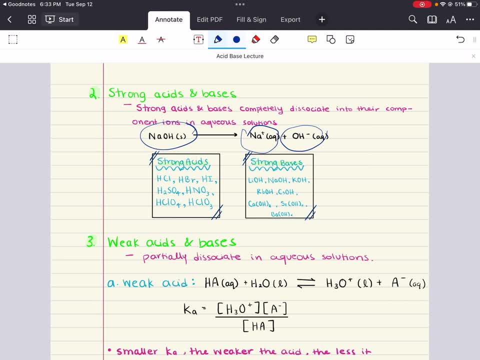 or base, such as sodium hydroxide, is added to water. So, for example, when sodium hydroxide is going to remain in solution. This is why the dissociation of strong acids and bases is set to go to completion. So in this sodium hydroxide example, all right, it's going to completely. 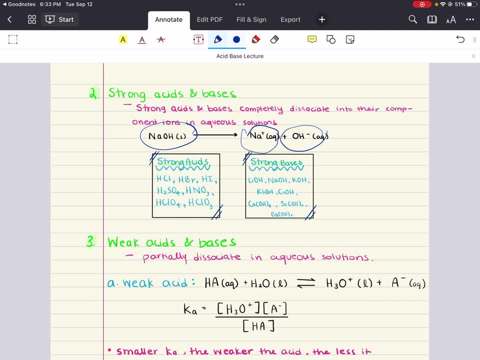 dissociate. We assume that the concentration of the hydroxide ions all right from the autoionization of water is negligible due to the addition of a strong base, And so the contribution of hydroxide and hydrogen ions from the autoionization of water is. 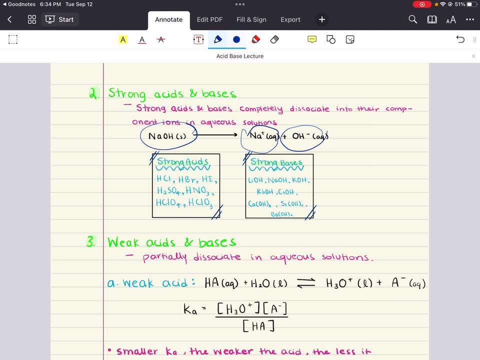 negligible if the concentration of the acid or base is significantly greater than 10 to the minus 7 molar. On the other hand, if the concentration of the acid or base is close to this or less than then, you would also factor in the contribution from the autoionization of water. all right It. 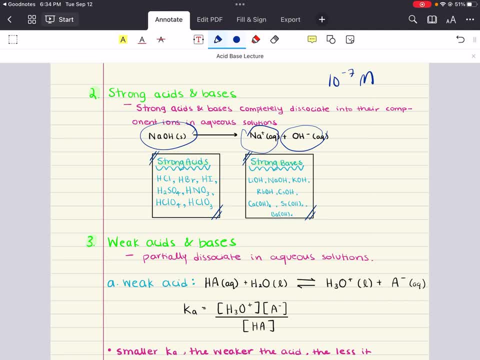 would be important in this case. Nevertheless, here is a list of strong acids and strong bases that I would recommend committing to memory for the MCAT. So our strong acids include chloric acid, hydrobromic acid, sulfuric acid, nitric acid, chloric acid, so on. 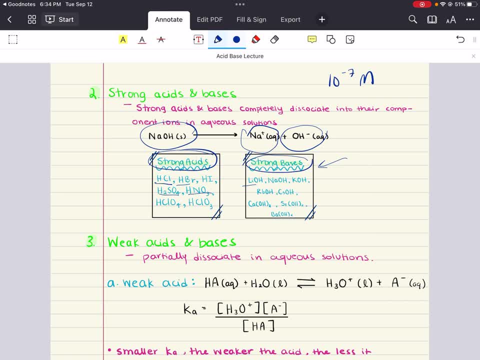 Strong bases: lithium hydroxide, sodium hydroxide, potassium hydroxide, calcium hydroxide, barium hydroxide, et cetera. all right, So we have a list of strong acids, list of strong bases. all right. Now what about weak acids and bases? all right. 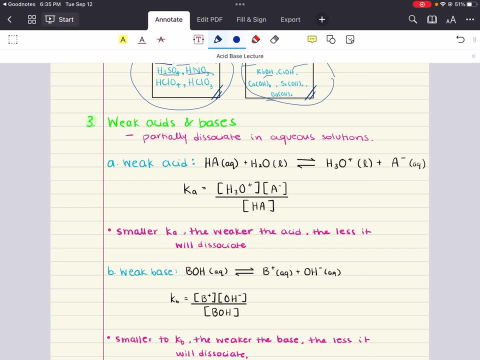 What's the difference, all right, between weak acids and bases and strong acids and strong bases? Well, a weak acid and base are acids and bases that only partially dissociate in aqueous solution. So a weak monoprotic acid like HA will dissociate. 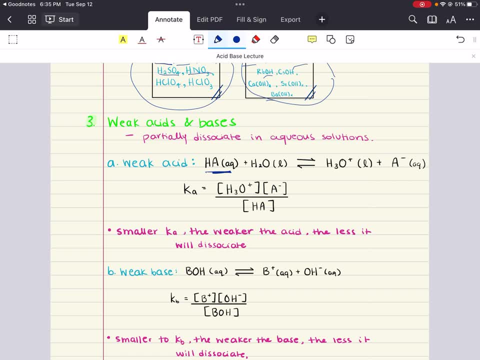 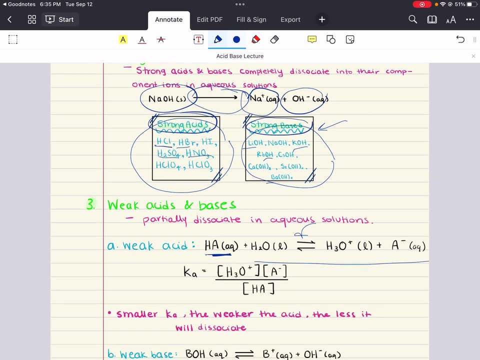 partially in water to achieve an equilibrium state that we can see here. all right. Notice, equilibrium state for strong acids and bases goes to completion, all right. So a weak monoprotic acid like HA will dissociate partially in water to reach an equilibrium state. Now, because the 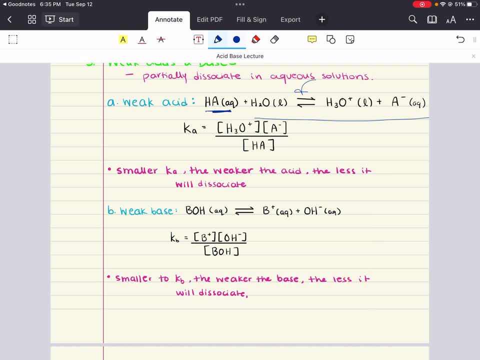 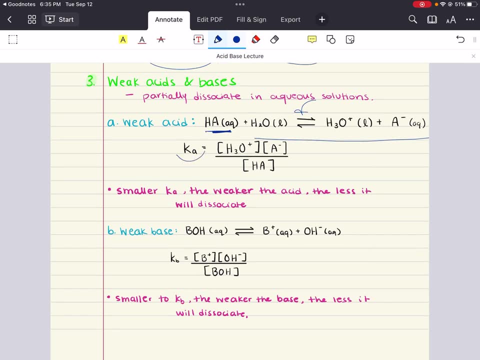 system exists in an equilibrium state. by the way, we can write the dissociation equation to determine the acid dissociation constant. all right, Remember, this is concentration of product over reactants. We only consider aqueous, or considering aqueous components only, all right. 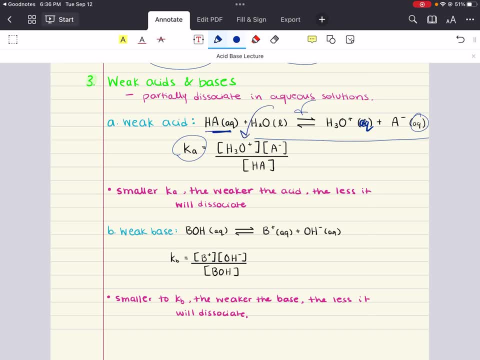 So we have Our hydrogen ions- our hydronium ions are our base, and then, of course, our weak monoprotic acid Cool. Sorry, by the way, this is supposed to say aqueous, not liquid, So that's just a. 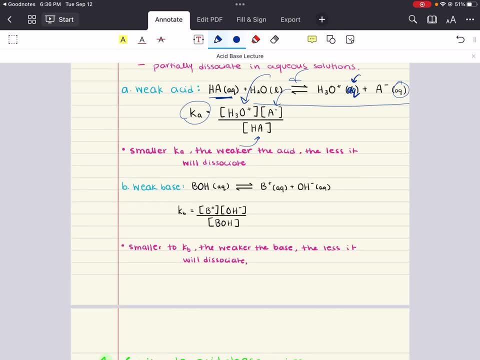 typo on my bad, all right. Then we have weak bases- all right. So a weak monovalent base like BOH, for example, undergoes also again partial dissociation to yield B plus and OH minus. again you see these equilibrium arrows because it only partially dissociates. And again here, 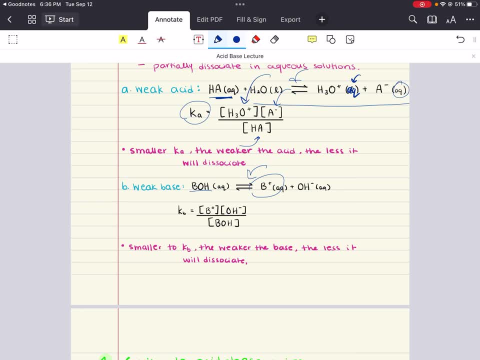 you can write a base dissociation constant. KB is going to be your concentration of your product over your reactants. Now, the smaller the KB. So some notes about KA and KB that are important For KA. the smaller the KA, all right. The smaller the KA, the weaker the acid. 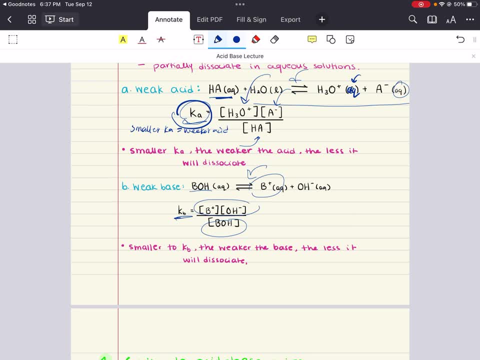 And consequently, the less it will dissociate, all right. What about KB, KB? the smaller the KB, the weaker the base, all right. And consequently, again, the less it will dissociate, all right. Now, generally speaking, generally, we can characterize a species as a weak acid if its 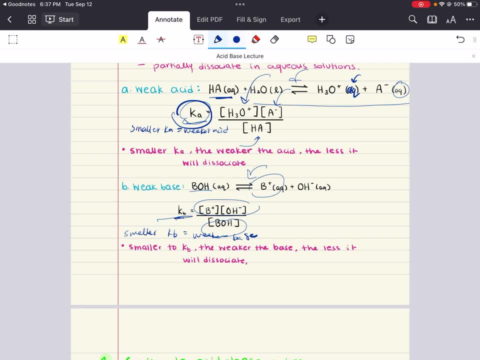 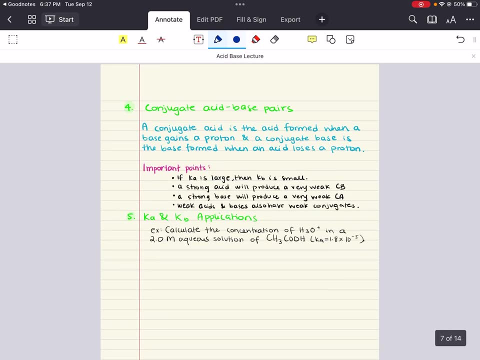 KA is less than one and a weak base if its KB is less than one. So we can characterize a species as a weak acid if its KB is less than one- Fantastic. The next thing we want to talk about is conjugate acid-base pairs. Now, because the Bronsted-Lowry definition of an acid-base reaction 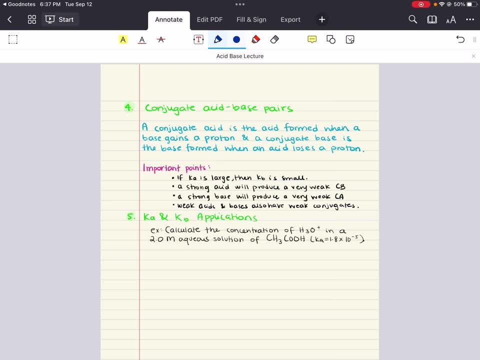 is one in which a hydrogen ion or a proton is transferred from an acid to a base. the two always occur in pairs called conjugates. So a conjugate acid is the acid formed when a base gains a proton, and a conjugate base is the base formed when an acid loses a proton. So, for example, we can write: 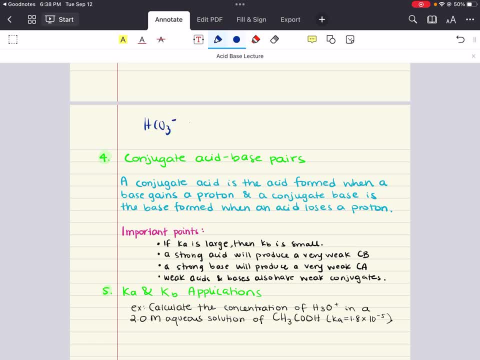 out HCO3- plus H2O, all right. This gives us CO2-3, CO3-2,- sorry, plus H3O+, All right. so what you notice is that this right here, all right, Is donating a hydrogen to water. So this is going to be the acid, This is going to be the 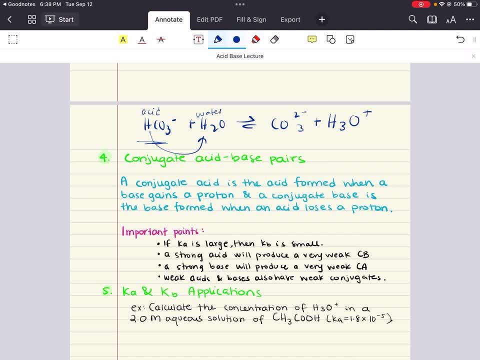 acid. Water is going to be the base, All right. now, when water gains a hydrogen, it forms hydronium ion. If water is the base, then hydronium ion is the conjugate acid. all right. And if this? 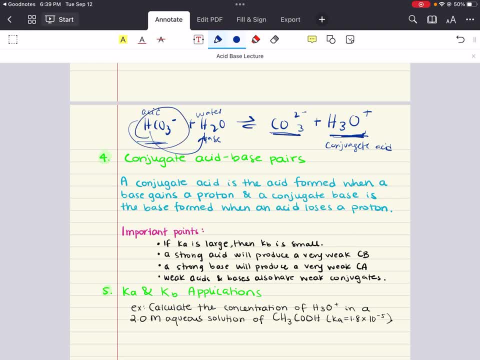 is the acid, then? what is formed when it loses a hydrogen is its conjugate base. all right, So a conjugate acid is the acid formed when a base gains a proton, and a conjugate base is the base formed when an acid loses a proton. All right, fantastic. Now some important points, Of course. 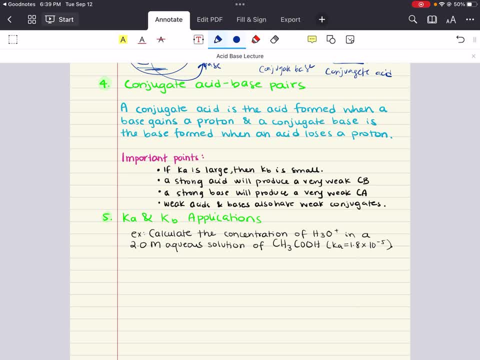 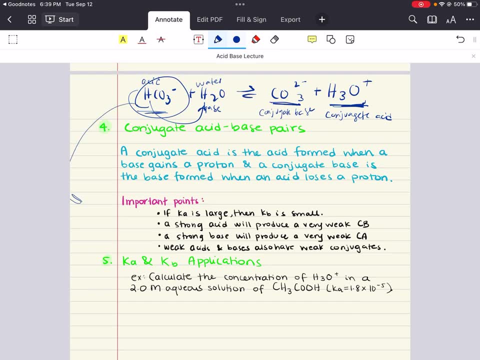 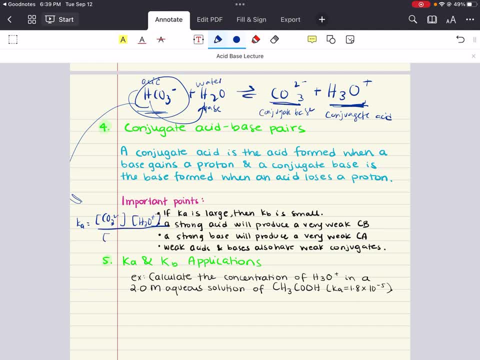 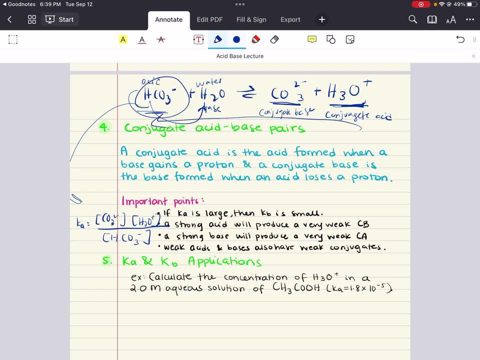 actually you can write. if you were looking at it this way, you can write Kb, all right. So forward Ka, backwards Kb. Some important things to keep in mind. if Ka is large, Kb will be small, all right. A strong acid will produce a very weak conjugate base. A strong base will produce a very 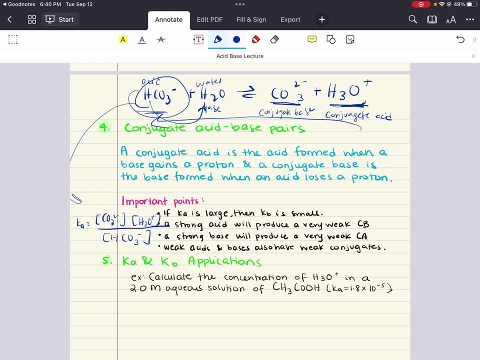 weak conjugate acid, and weak acids and bases also have weak conjugates. all right Now to really put into effect our conversation on acids and bases, and specifically Ka and Kb, let's tackle a practice problem together, all right. So this problem says: calculate the concentration of H3O? 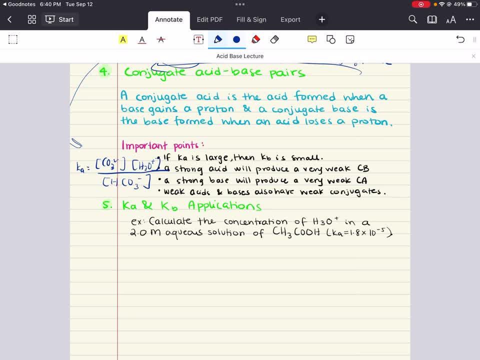 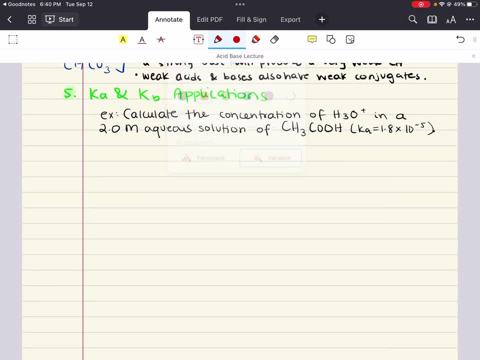 plus in a 2-molar aqueous solution of acetic acid, and they give us the Ka value- Fantastic. So the first thing we want to do, all right, is write out the equation for this acid: acetic acid, CH3COOH in water, All right. 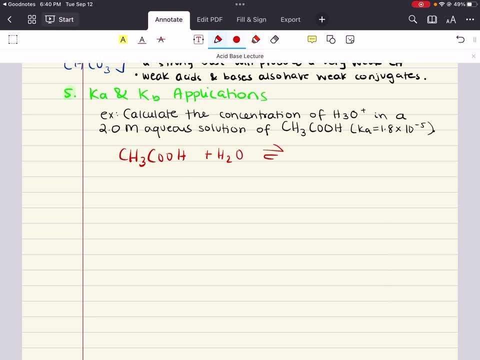 This is the acid, hence the name acetic acid. So it's going to donate a proton to water, And so we're going to have acetate, CH3COO minus, plus hydronium ion, CH3O plus. All right, And we can. 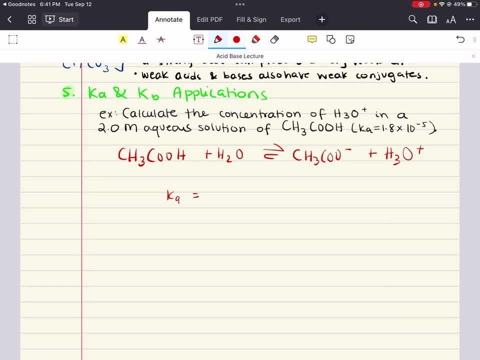 write the Ka. Remember it's the concentration of the product over the reactants, only the aqueous species, which is just going to be our acetic acid, our acetate and our hydronium. All right, Water is a liquid, Fantastic. So we don't include that. So it's going to be H3O plus, All right. 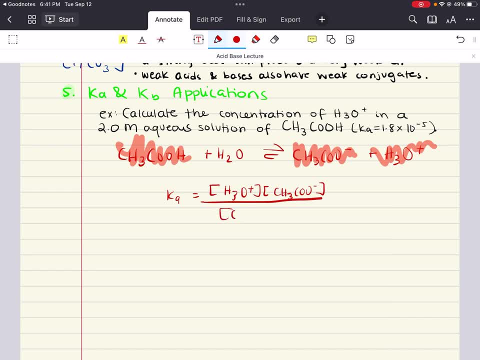 CH3COO minus all over CH3COOH. All right, And this is equal to- we're given the Ka value. So 1.8 times 10 to the minus Five. Now we want to recognize that acetic acid is a weak acid And you would know that if you had. 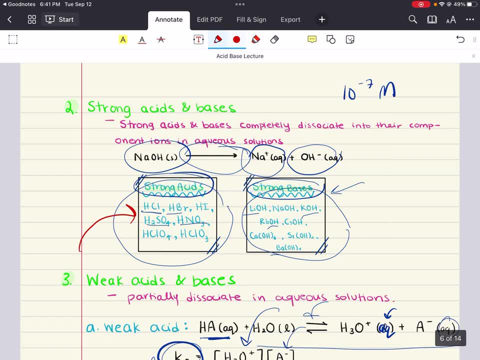 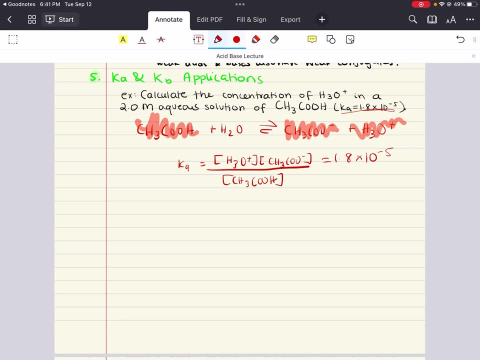 if you have, if you have your strong acids memorized because you realize that acetic acid is not on that list, All right. So acetic acid is a weak acid. So the concentration of acetic acid at equilibrium is going to be equal to its initial concentration to molar. 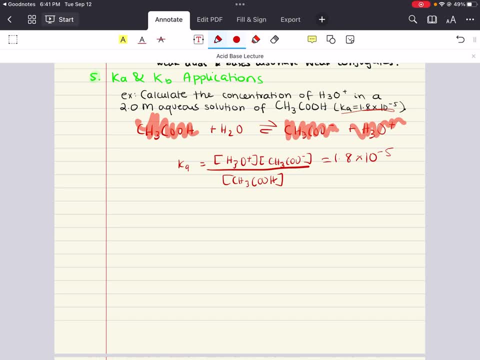 minus the amount dissociated, So X, All right. Likewise, the concentration H3O plus is going to be equal to that concentration of CH3COO minus, which is going to be equal to X, because each molecule of acetic acid dissociates into one hydrogen ion and one. 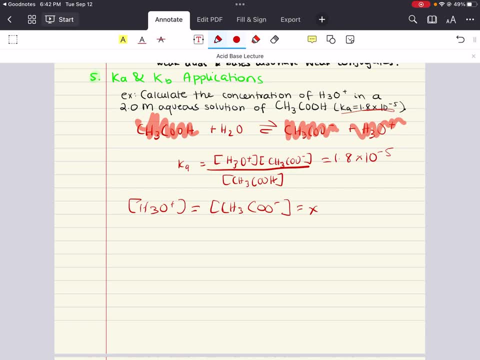 acetate ion. All right. Also something else to note. Note that the contribution of hydronium ion from water is negligible, And so that means All right. What we can write is that Ka is equal X times X over two molar minus X. All right, Just like we noted, we said, acetic acid is a weak 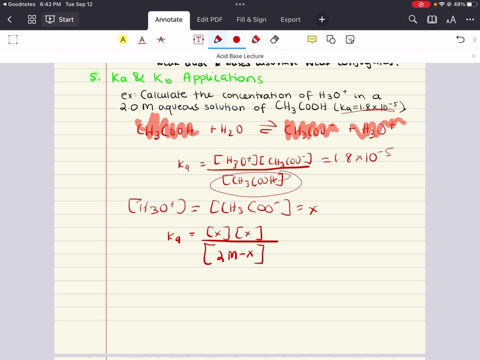 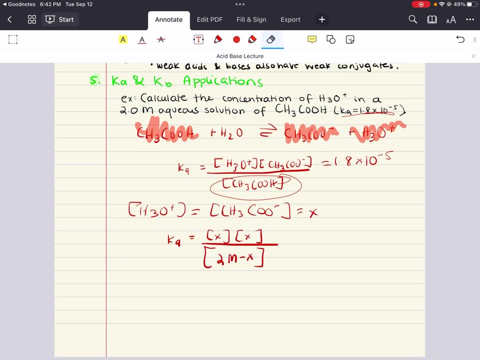 acid, And so the concentration of acetic acid at equilibrium is equal to its initial concentration minus the amount dissociated. So that's why we write two molar, All right, Minus X, And I'm just going to erase the molar. So we're just looking at two minus X for now. And again we said: 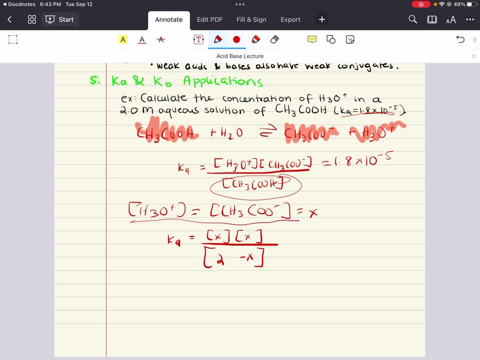 that the concentration of these ions are the same. They're going to be equal to X, because each molecule of acetic acid dissociates into one hydrogen ion, one acetate ion, And so now we have this equation that is equal to the Ka 1.8 times 10. 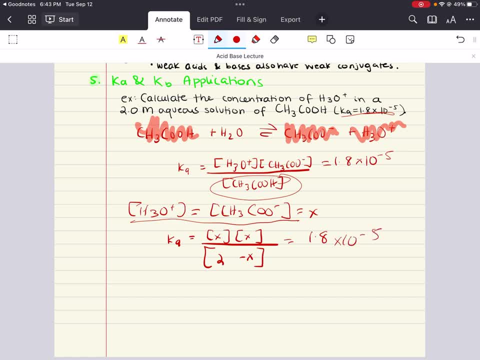 to the minus five. All right, Now here's something. Remember that the value of X is generally very small, And so, therefore, we can actually approximate this two minus X to just approximately two. All right, And so what we're going to have in the numerator is X squared. 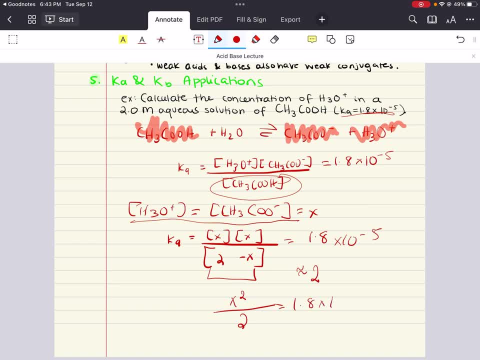 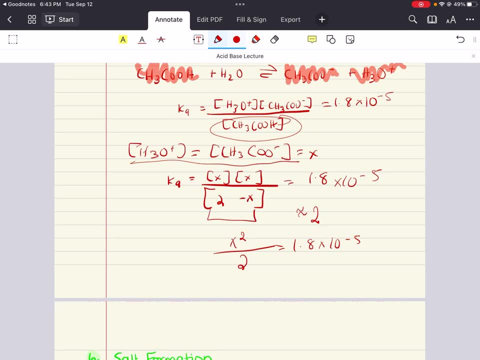 In the denominator two and that's going to be equal to 1.8 times 10, to the minus five, All right. And, by the way, X is generally very small And this is further supported because acetic acid is a weak acid and only slightly dissociates in water, So it makes sense to make. 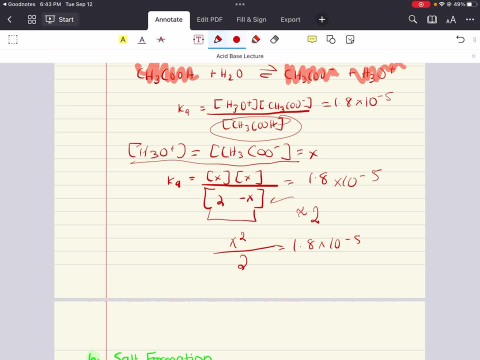 this approximation. Now we have X squared over two equals 1.8 times 10 to the minus five. All right. We can multiply both sides by two, All right. And then square root both sides, All right. And for X we're going to get six times 10 to the minus three molar. Now again, 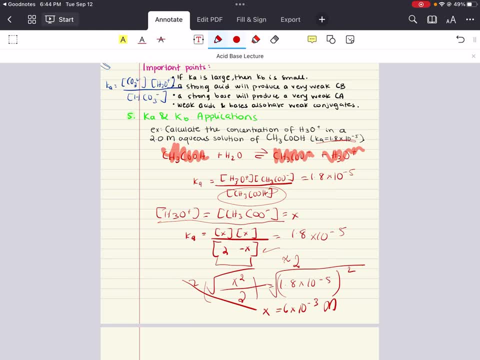 I want to preface this- that during lectures we do mathematically harder problems so that we can understand the concepts. All right, This will generally be easier in regards to math on in the problem set and what you're more likely going to encounter in the MCAT. Even then, we can make the 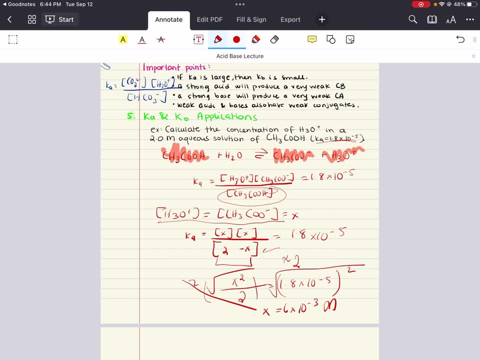 argument that you know multiplying both sides is by two is not that hard. One point eight, two is just three point six, All right Times 10 to the minus five. And actually you can go ahead and move the decimal and say 36 times 10 to the minus six and 36. 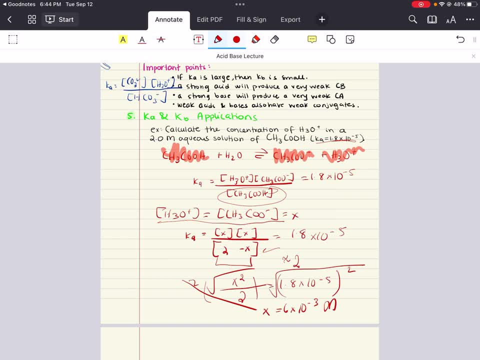 is a perfect square, So you can easily do the square root of that. Hence why we got six times 10 to the minus three. All right Now. this X represents the concentration of H3O plus. So the concentration of H3O plus is equal to six times 10 to the minus three. 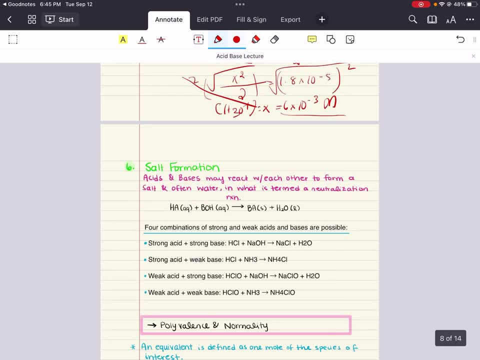 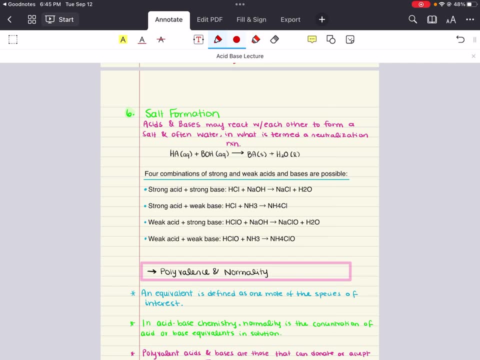 molar Beautiful. Now we can move to our final topic in this objective, All right, And that is salt formation. Acids and bases may react with each other to form a salt and often, but not always, water in what's termed a neutralization reaction. So, for example, we can write the following: 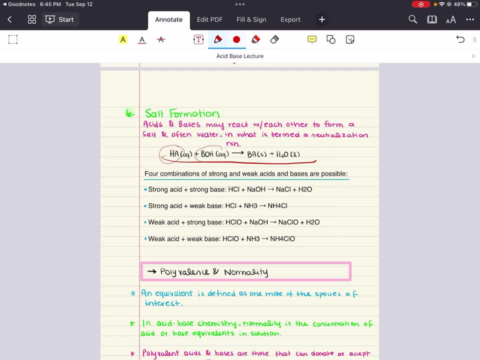 expression right here. Have acid react with a base, It's going to form salt and sometimes water. Now the salt may Precipitate out or remain ionized in solution, depending on its solubility and the amount produced. In general, neutralization reactions go to completion. The reverse reaction, in which 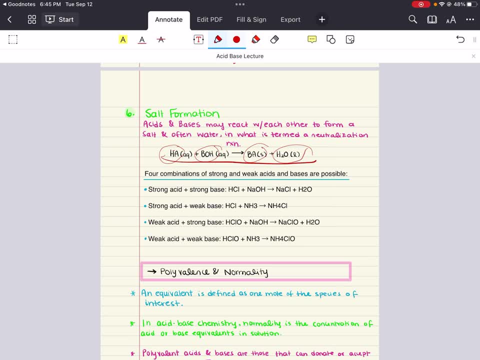 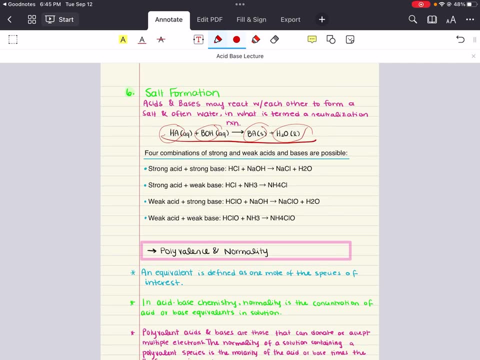 the salt ions interact with water to give back. the acid or base is known as hydrolysis. Now there are four combinations of strong and weak acids and bases that are possible. You can have strong acid and strong base, like we see here. You can have strong acid and weak. 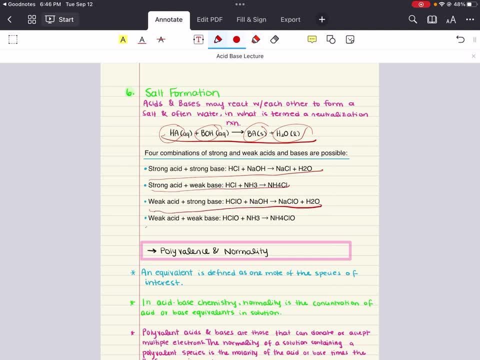 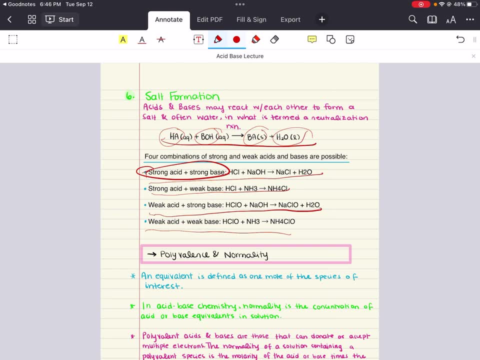 base. like you see here, Weak acid and strong base or weak acid and weak base. Now the product of a reaction for a strong acid, strong base are equal molar amounts of salt and water. The acids and bases neutralize each other, So the resulting solution is neutral, So it usually has a pH. 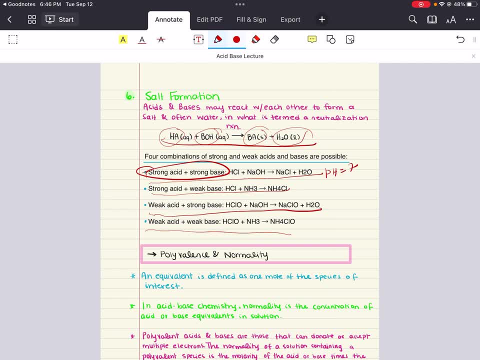 equal to seven, And the ions formed in the solution will not react with water because they are inert conjugates. Now the product of a reaction between a strong acid and weak base is also salt, but often no water will be formed because weak bases are often not hydroxides. 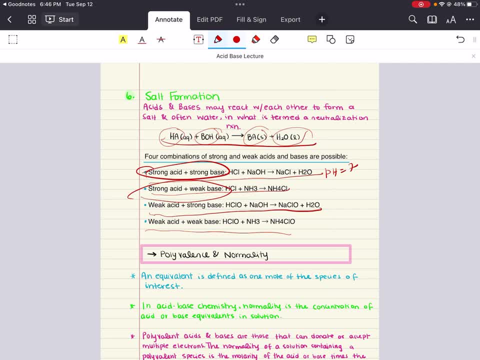 In this case, the cation of the salt is a weak acid and will react with the water solvent, reforming some of the weak base through hydrolysis, All right. And then, on the other hand, we have weak acid and strong base. The pH of the solution at equilibrium is going to be within. 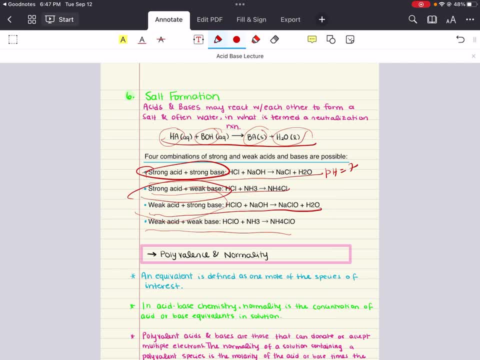 the basic range because the salt hydrolyzes with concurrent formation of hydroxide ions. The increase in hydroxide ion concentrations is going to cause the system to shift away from autoionization, thereby reducing the concentration of the hydronium ions And, consequently, 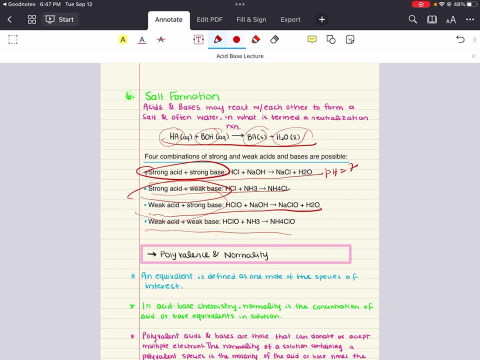 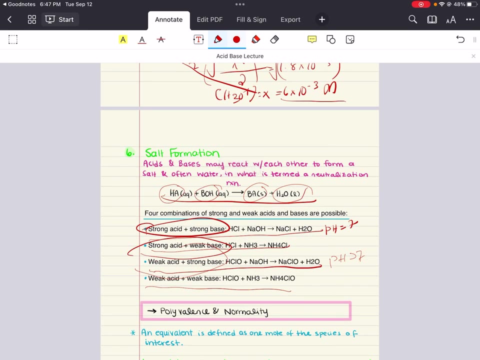 the concentration of the hydroxide ion will be greater than that of the hydronium ion at equilibrium, And so, as a result, the pH of the solution will usually rise above seven. for something like this, All right, Fantastic. That is objective one and objective two that we have. 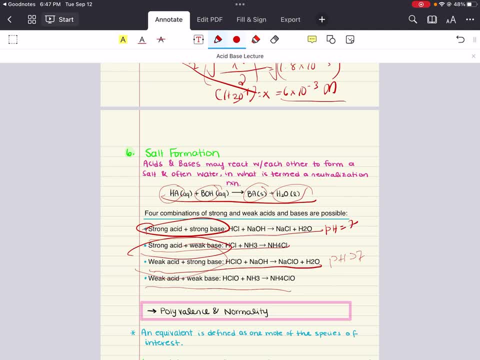 covered. All right, Please let me know if you have any questions. comments concerns: We were able to cover definitions of Arrhenius acids, Arrhenius bases- We said Arrhenius acids dissociate to produce an excess of hydrogen ions in solution- and Arrhenius bases Just as a review. 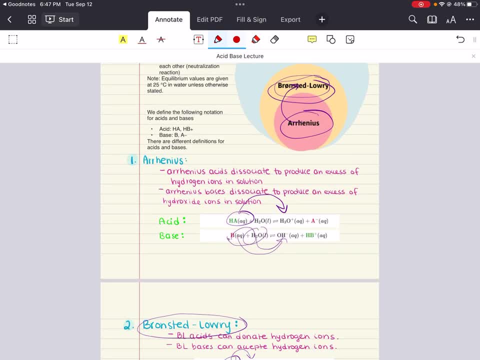 sorry, I just started talking without telling you. Let's do a quick review. Let's do a quick review. Arrhenius acids: they disassociate to produce an excess of hydrogen ions And solution. Arrhenius bases: they dissociate to produce an excess of hydroxide ions and solutions. 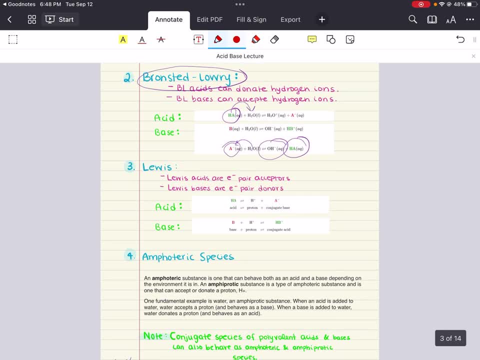 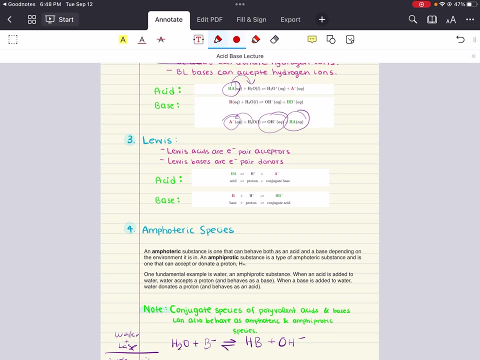 Then we talked about Bronsted-Lowry definitions. Bronsted-Lowry acids are species that can donate hydrogen ions. Bronsted-Lowry bases are species that can accept hydrogen ions. Lewis acids are electron pair acceptors. Lewis bases are electron pair donors. Now all Arrhenius acids. 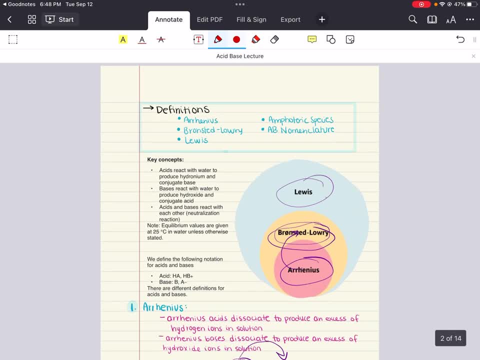 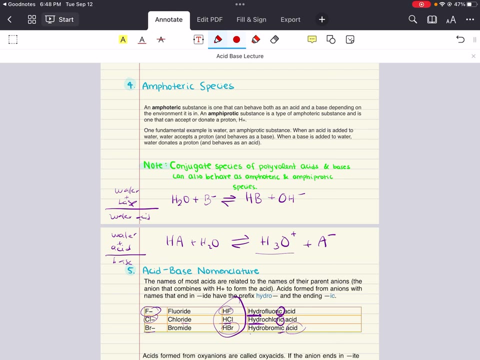 and bases are Bronsted-Lowry acids and bases, And all Bronsted-Lowry acids and bases are Lewis acids and bases. However, the converse of the statements is not necessarily true. Then we talked about amphoteric species. Those are species that can behave as an acid.